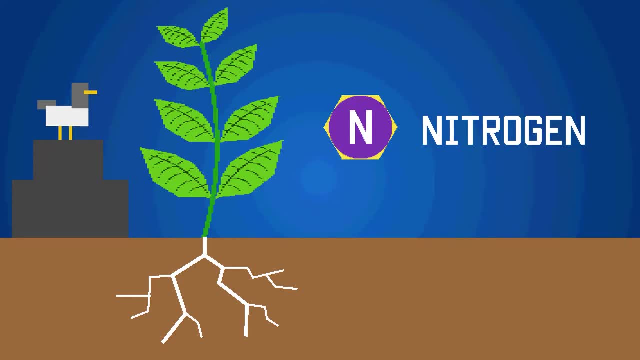 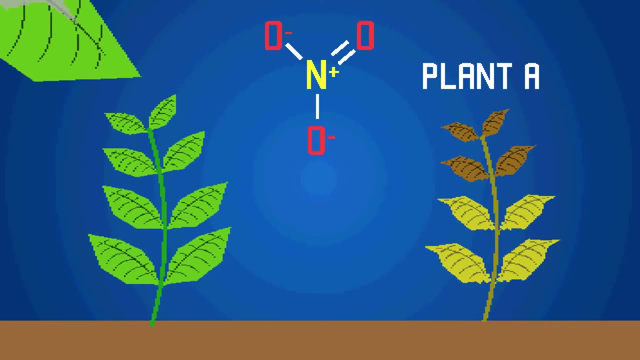 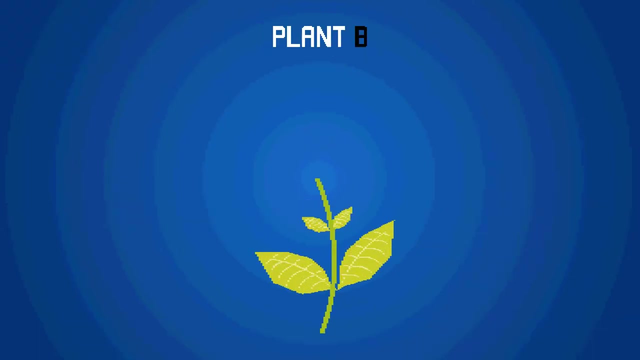 nitrogen is needed to make protein. Plant A has not obtained enough nitrogen, which it should get by absorbing nitrate ions from the soil. As you know, nitrogen is needed to make protein, So without this element, the plant will have stunted growth. The older leaves will be yellow and sometimes shriveled. Take a look at. 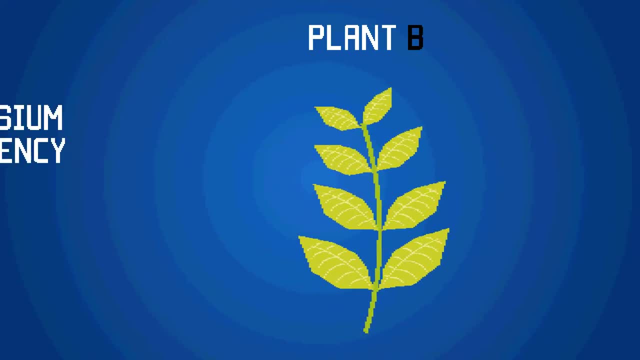 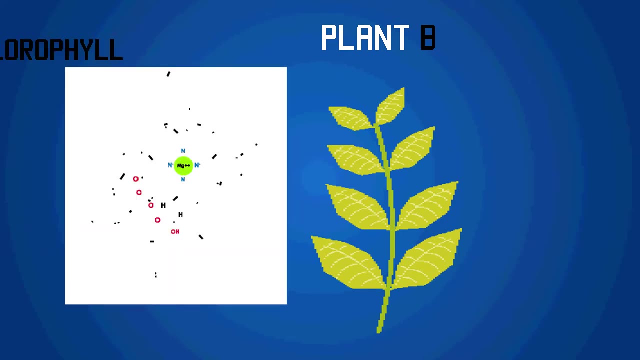 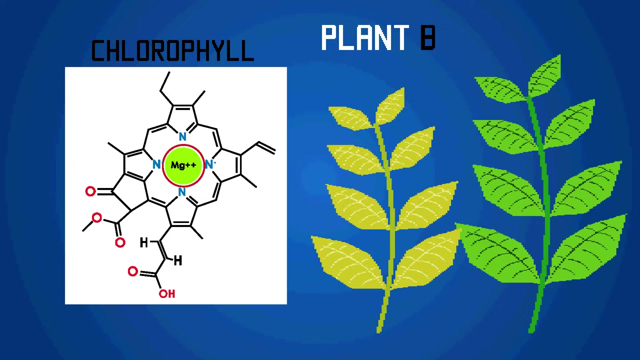 poor plant B. This plant has a magnesium deficiency. As you can see, it is yellow. This is because magnesium is needed to make chlorophyll, the green pigment that absorbs light in chloroplasts. As this plant does not have enough chlorophyll, its growth will be limited, as it will do less photosynthesis. 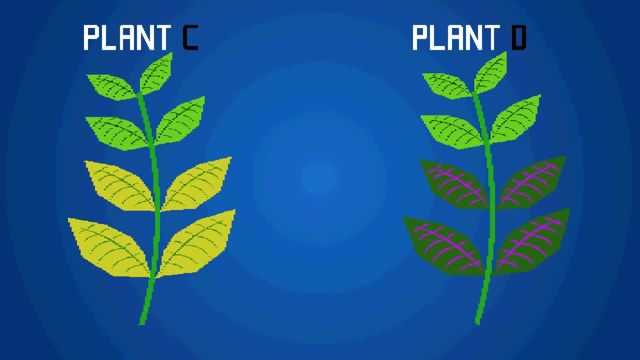 Now let's look at plants C and D. They are also both suffering from nutrient deficiencies. Why don't you pause the video here and write down any differences you see between them? Plant C had a potassium deficiency. The older leaves are yellow, but the veins 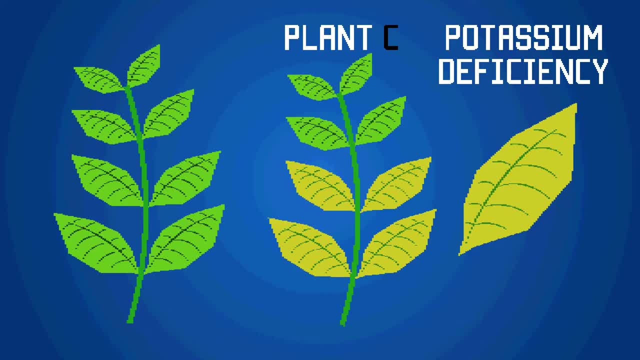 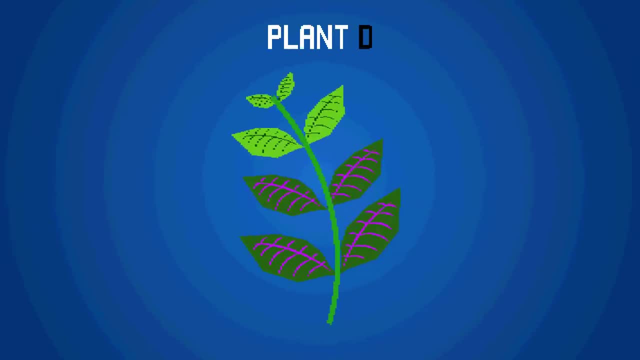 remain green. The plant is also not growing properly. Potassium is needed for growth and for the plant's immune system. Plant D has a phosphate deficiency. The older leaves are darker green and some have fallen off. Sometimes the veins become purple and the plant's growth has also been stunted. 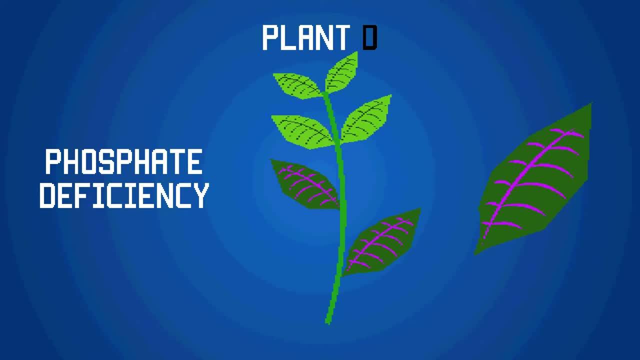 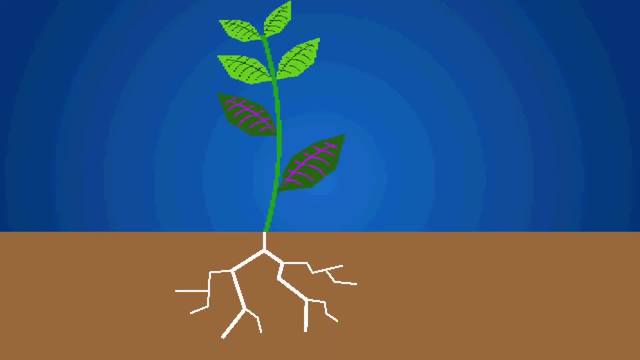 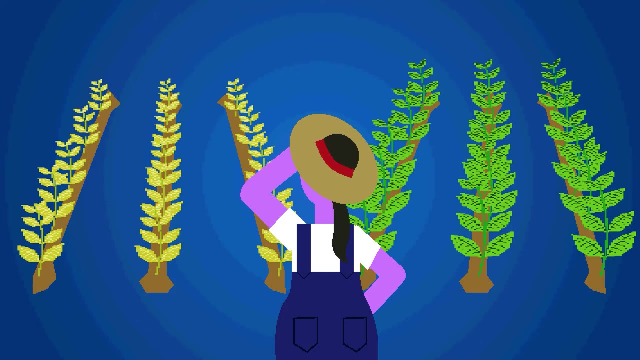 This is because phosphorus is involved in energy transfer, so the whole plant won't grow correctly, including the roots. Nutrient availability is of crucial importance for farmers, as plants without all of the nutrients they need will grow slower and produce smaller yields, like less fruit. Hydroponics is a new type of agriculture where plants 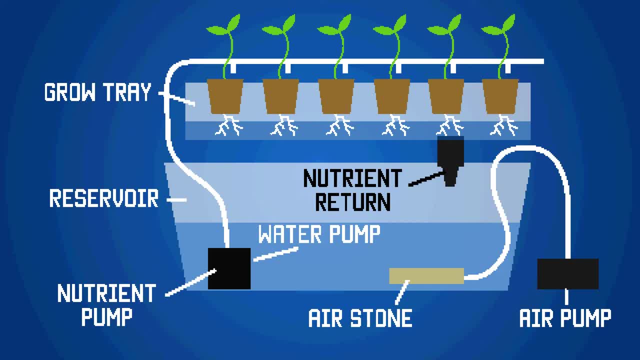 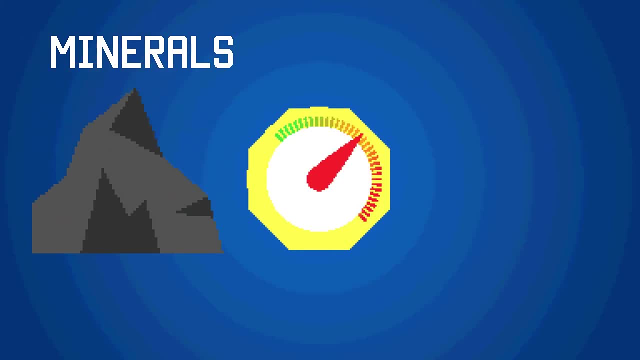 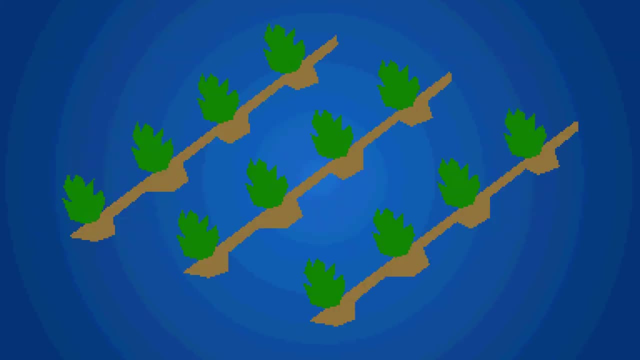 are not grown in soil. Instead, their roots are suspended in water with nutrients. This way, the farmer has much more control over the minerals in the solution the plants grow in. In traditional farming, where crops are grown in soil, the farmer may use crop.